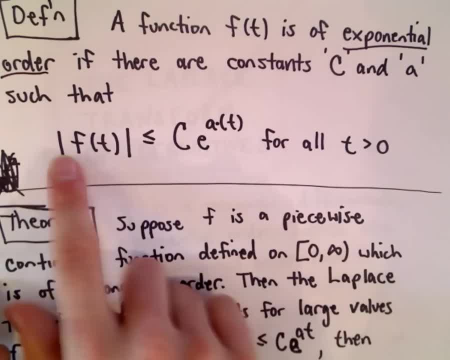 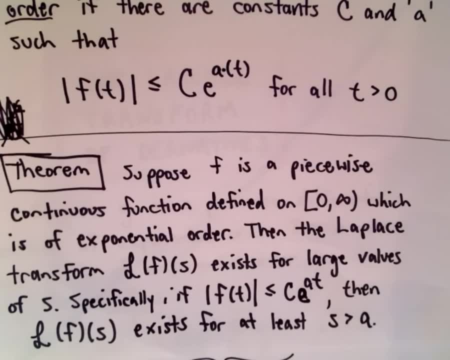 I mean exponential functions get really big, really, really fast. So this is kind of good in the sense that there are lots of functions of exponential order. Another little theorem here: Okay, so suppose f is a piecewise continuous function, and I didn't give the definition of piecewise continuous. 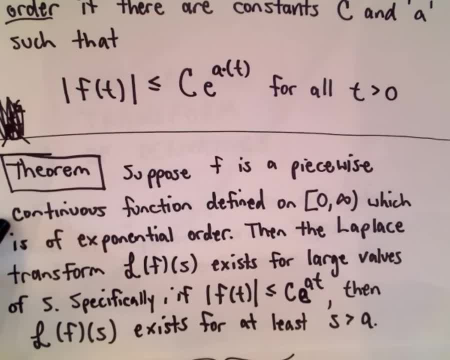 but we say a function is piecewise continuous if it has only finitely many points of discontinuity over any finite interval. and at every point of discontinuity the limit of f exists from both the left and the right. Okay, so you may. 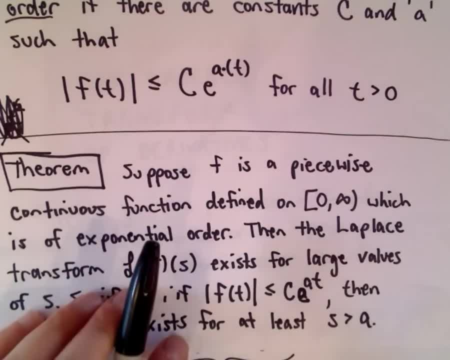 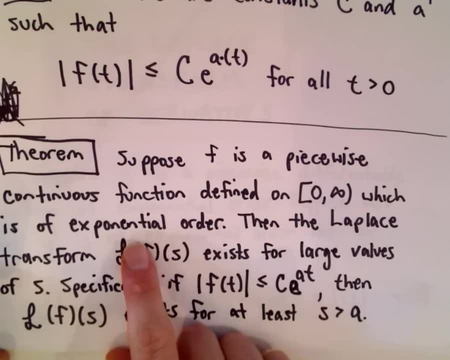 you may look up piecewise continuous function. I forgot to write that one down. but if you've got a piecewise continuous function defined on zero to infinity and that function's of exponential order, it says the Laplace transform exists. basically is what it says. 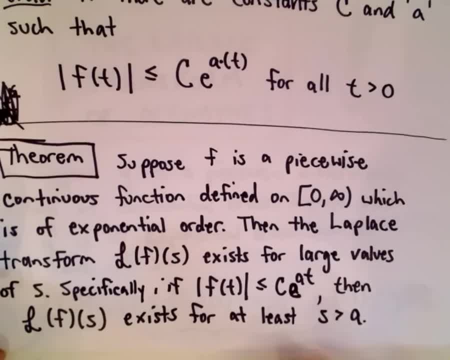 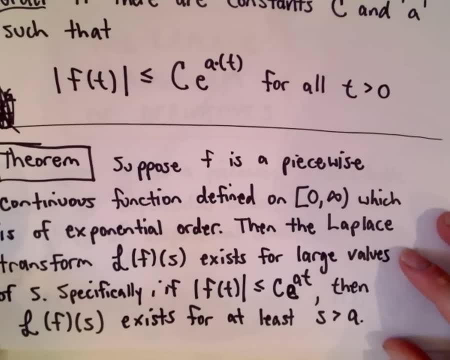 Okay, so that's what you need to take away from this theorem. If you have a piecewise continuous function, it's of exponential order. well, then you can start using Laplace transform stuff on this. Okay, Again, not all functions are of exponential order. 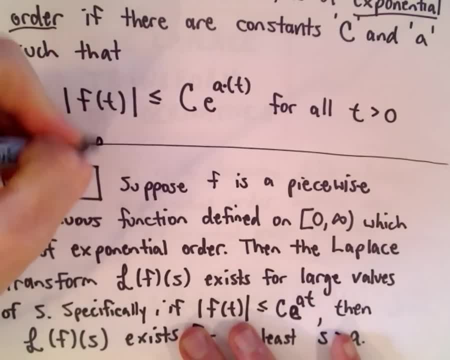 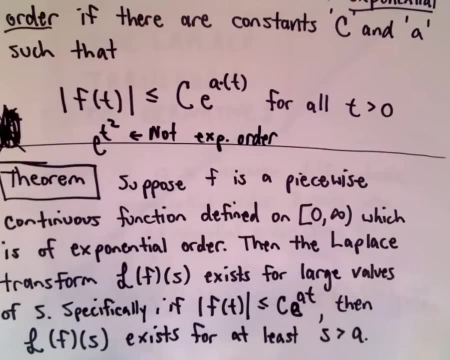 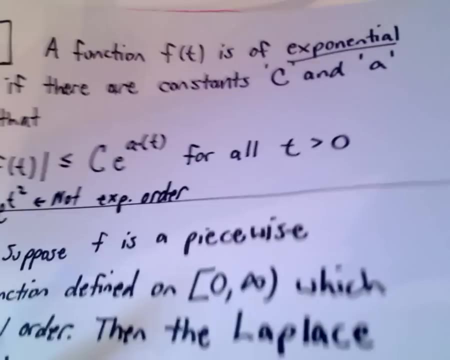 I kind of, I think, scratched one out here. For example, e to the t squared, that would be not of exponential order- just to throw out a function that you know wouldn't satisfy this stuff, for example. Alrighty, so a couple definitions here. 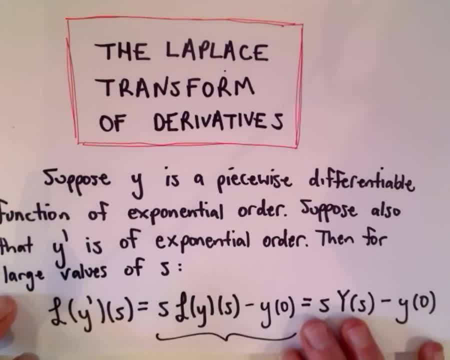 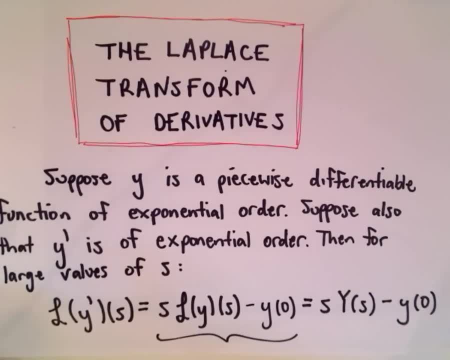 So the next thing I want to talk about here is kind of the important, one of the big, important properties to use in order to solve these differential equations using Laplace. So what it says is: it says: suppose y is a piecewise differentiable function. 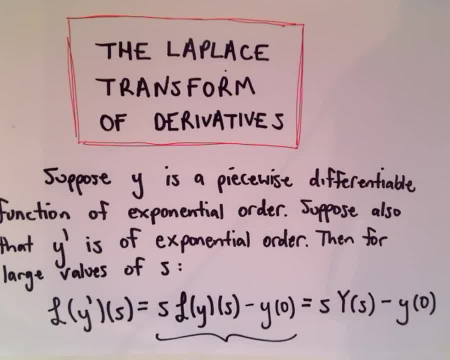 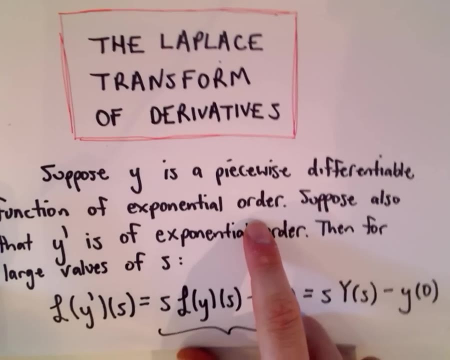 and I guess I didn't give piecewise differentiable either. but we say a function is piecewise differentiable if it's continuous and if its derivative is piecewise continuous. So again a couple definitions maybe to look up. So if it's piecewise differentiable and of exponential order, and also suppose its derivative is of exponential order. 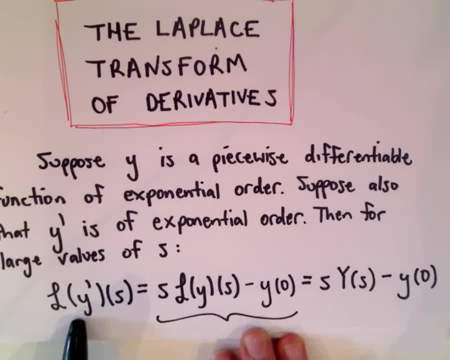 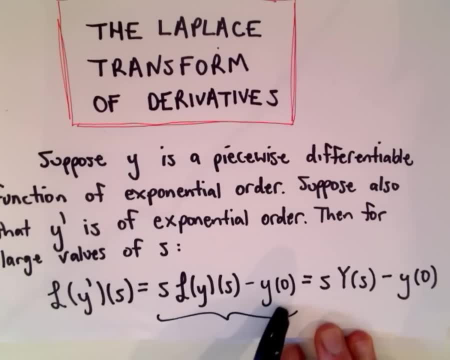 then what it says? basically, it says the Laplace transform of the derivative is going to equal s times the Laplace transform of the original function, minus this initial condition y of 0.. Okay, and just alternate notations here, for again for the Laplace transform. 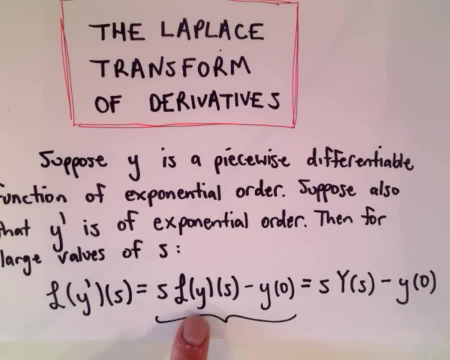 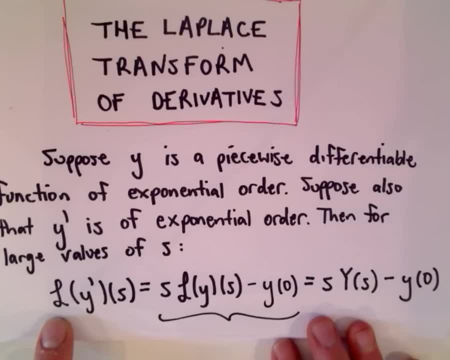 So what this really kind of says, if you think about it you know normally having a function and taking its derivative, that can be kind of a tedious process. but it says under the Laplace transform somehow taking the derivative is somehow equivalent to. 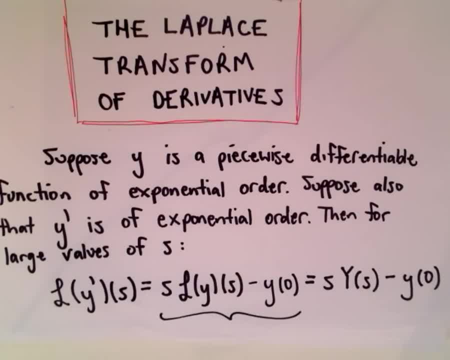 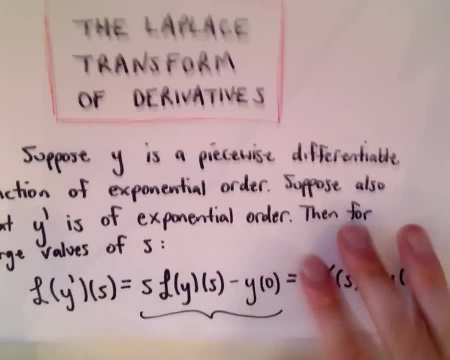 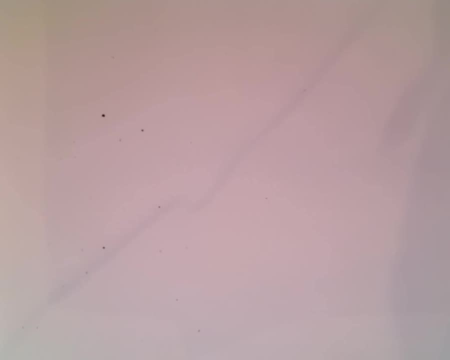 multiple multiplying by s under this Laplace transform. So somehow this just makes things mechanically much easier to deal with. All right, well, let's prove this. Let's prove this since it's so important. So take here, you know, a couple minutes to go through this proof. 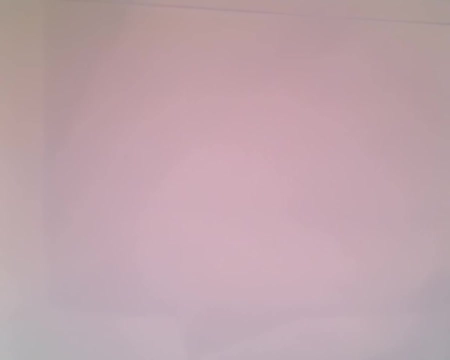 Again, all we're really using is integration by parts, So that proposition is the important thing. Again, if you're just wanting to see the mechanics, you could probably skip this proof, But again, I think it's kind of just, you know, insightful as to what's going on. 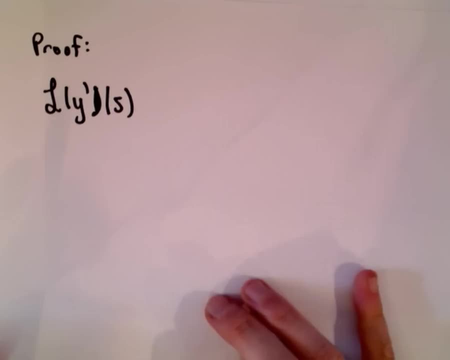 Okay, so we've got the Laplace transform of the derivative of s. Well, by definition that's just the integral from 0 to infinity, y prime of t. so we take our function e to the negative st dt. 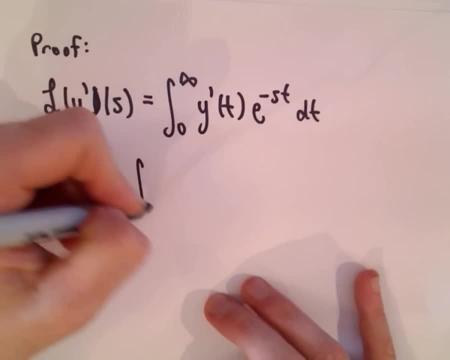 And well, this is just one of these nice little improper integrals. So I'm going to use 0 to capital T and then we'll have the limit as t goes to infinity. So we've got y prime of t, e to the negative st dt. 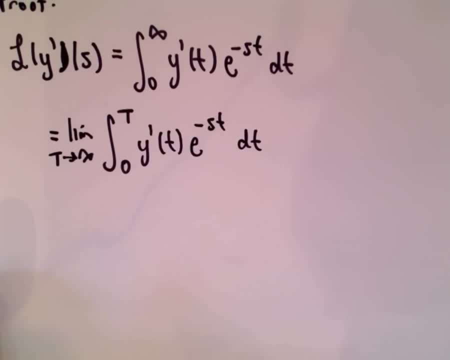 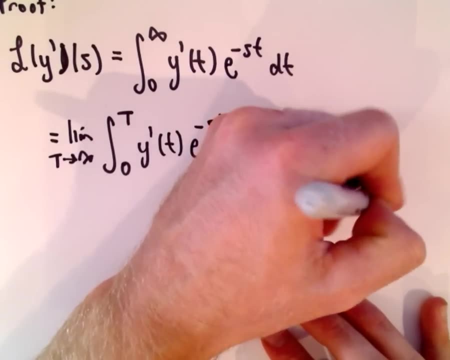 So now we've got to integrate this lovely function And you know, again, we're just going to use integration by parts on this. So the integral of u dv is uv minus the integral of v du. Let's see here: 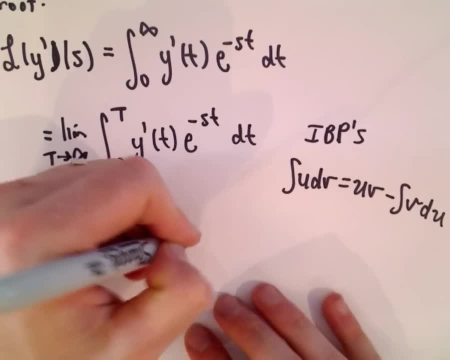 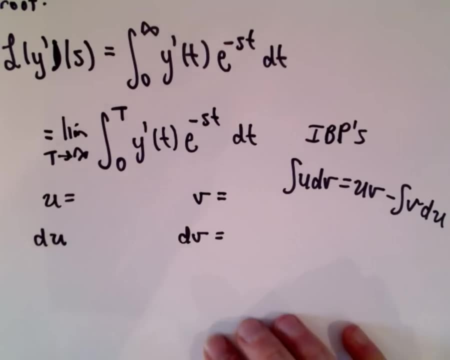 So we've got to pick u and from that we'll calculate du. We'll pick our dv and from that we'll integrate. to get back to v, Well, I'm going to let dv be the derivative portion, the y prime of t, dt. 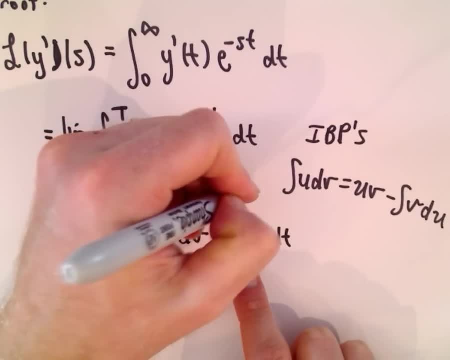 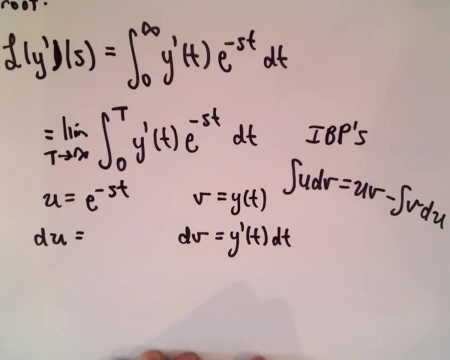 Well, if you integrate that, if you integrate the derivative, we'll just get back to our function y of t. So that means we'll let u be the e to the negative st portion, And when you take the derivative we get e to the negative st, But then by the chain rule. 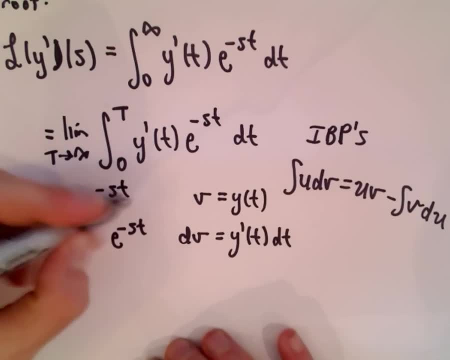 you've got to multiply by the derivative of the exponent. Since t is our variable, that means we'll pick up a negative s. Okay, I'm trying to separate that there a little bit, Alright, so now we're just going to fill in. just use our integration by parts. 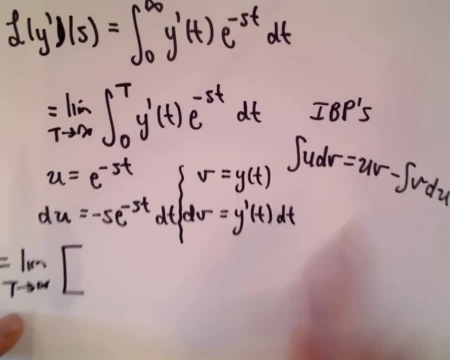 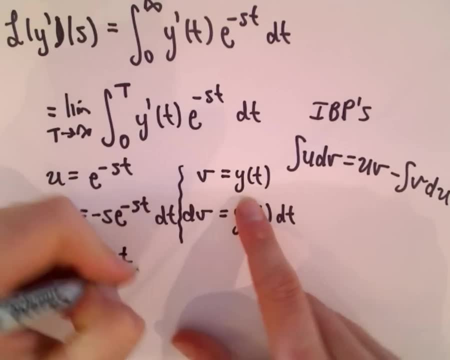 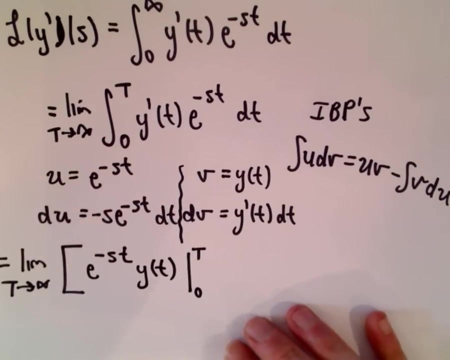 formula. So we have the limit as t goes to infinity. So it says: well, you get u times v, So u times v, so we have e to the negative st times y of little t. Our limits of integration would be zero to capital T. 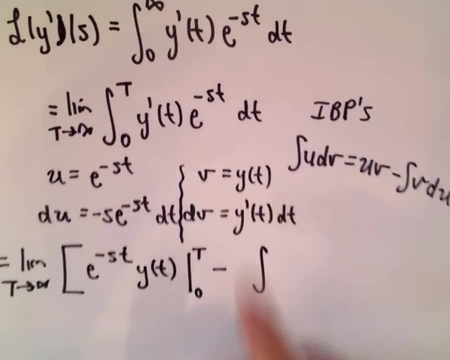 Minus the integral of v okay, which is y of t times du, which is negative s e to the negative st. This negative s is a constant, though, so I think I'm going to factor that negative s out front, and that'll give us: 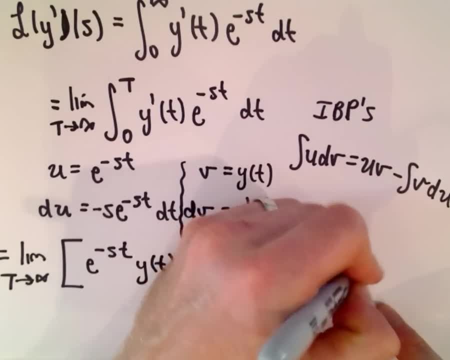 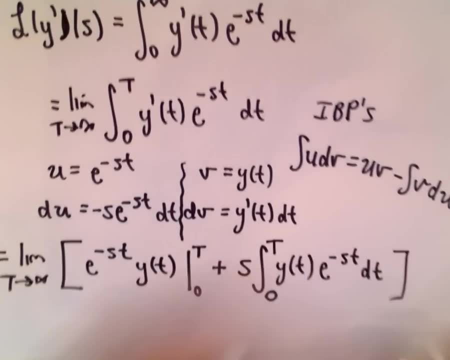 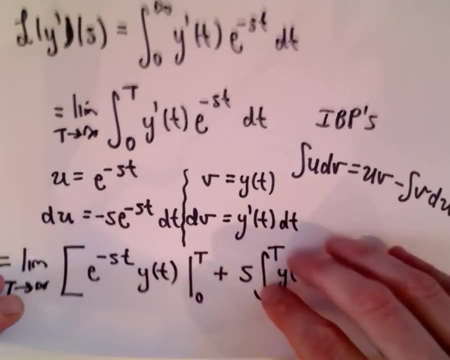 well, positive s. Then we have e to the negative st, dt. Again, our limits of integration: zero to capital T. Alright, so getting a little bit, uh, a little bit closer here. So now all I'm going to do is just start plugging in. 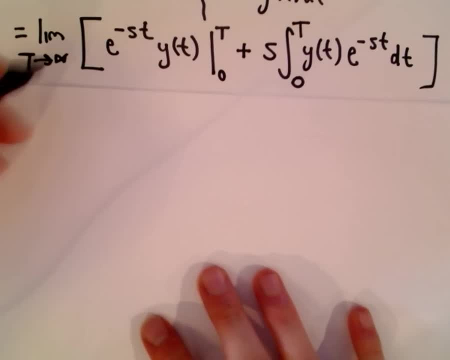 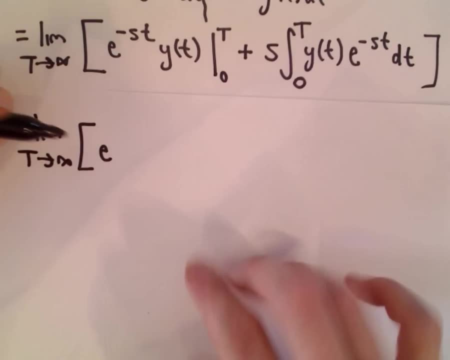 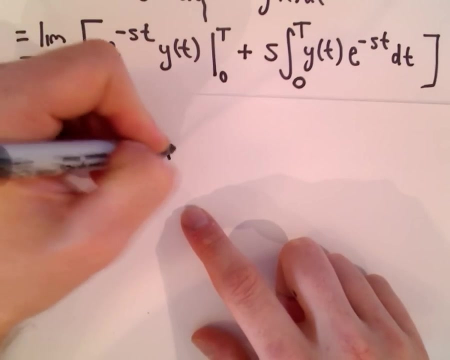 limits of integration. Okay, so it says we've got the limit as capital T goes to infinity. So again we're replacing. remember little t's are variables. so we'll get e to the negative s times capital T and then y of capital T. So when I plug in the 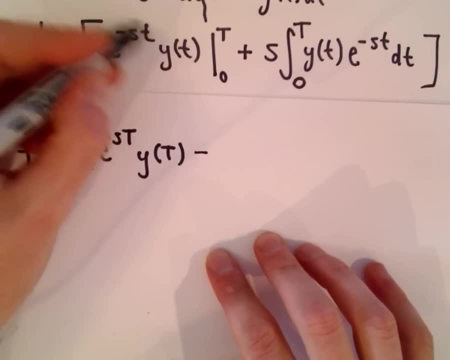 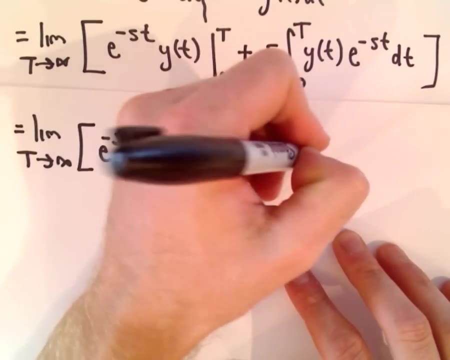 upper limit minus. let's see when we plug in uh zero, well, we'll get e to the zero times y of zero, And I'm going to leave this other part alone. here It's from zero to t, y of t. 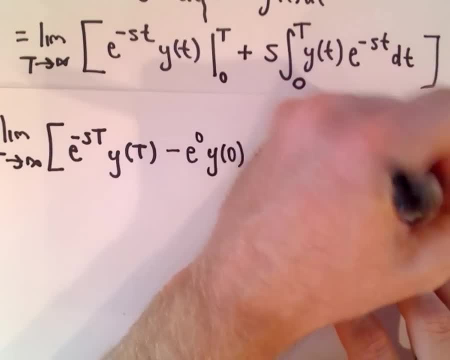 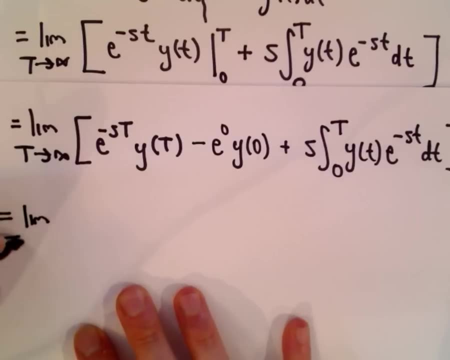 e to the negative st dt. Well, okay. so if you think about it, you know, if you apply the limit, we've got well the limit, as t goes to capital infinity, and then we have well the limit, as t goes to capital infinity, and then we have well the limit, as t goes to capital infinity, and then we have well the limit, as t goes to capital infinity. 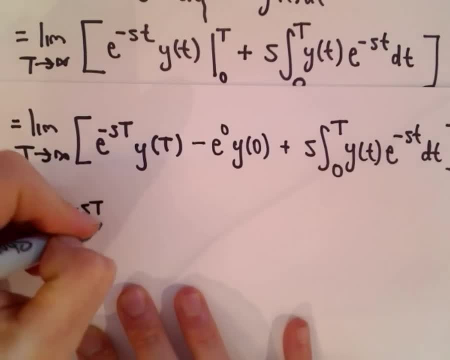 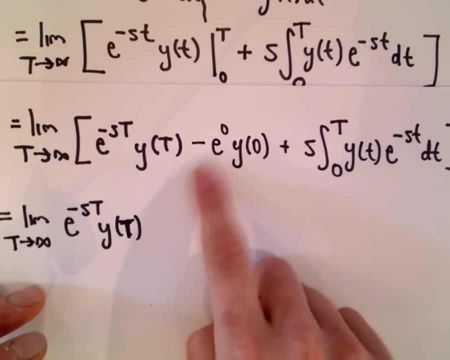 We've got e to the negative st y of t. Notice the middle part's just actually going to be a constant. e to the zero is one. y of zero is just the- you know- initial condition associated with the original function. 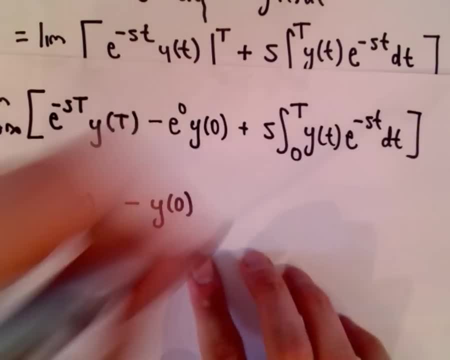 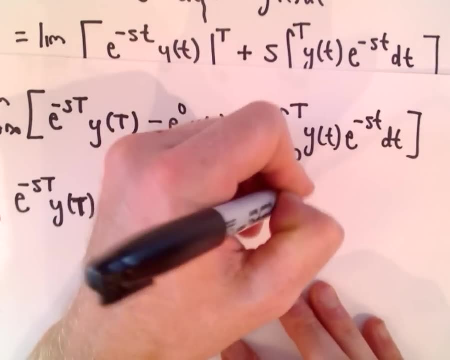 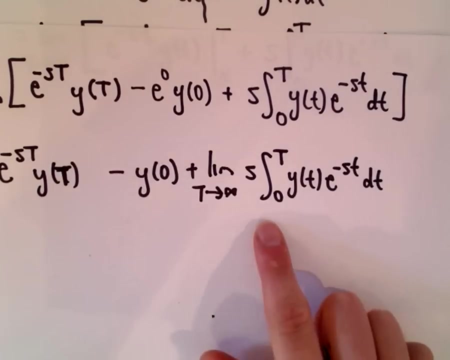 So we'll just get minus y of zero, And then we would have the limit as t goes to infinity of s times, zero to t, y of t, to the negative ST DT. but notice now this, this, this portion from 0 to T as T. 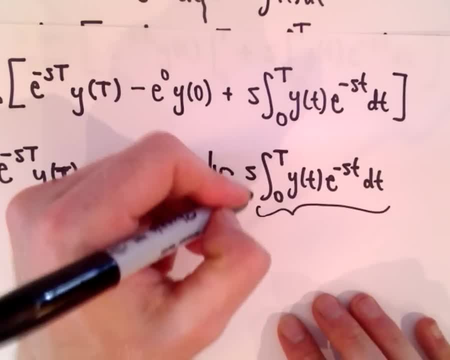 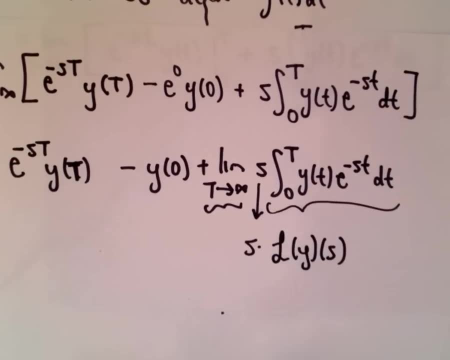 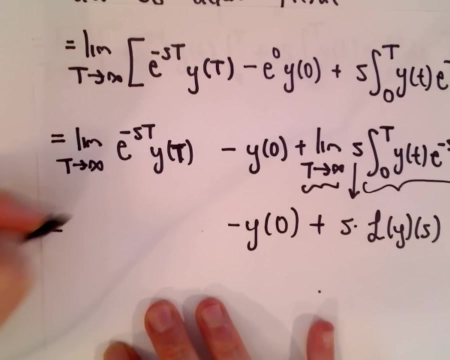 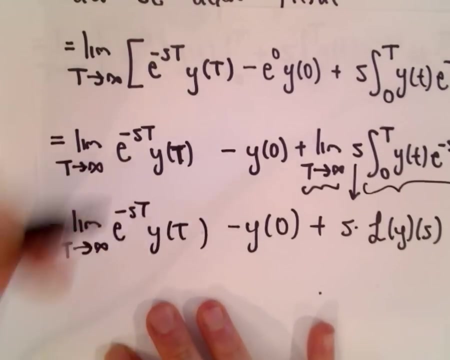 goes to infinity. that's just the Laplace transform of the original function being multiplied here by S. all right, so I'm getting a little bit closer here. so now kind of the question is, what happens to this first term? so that's the only thing where we really still have the limit, the limits still hanging out. so now we have 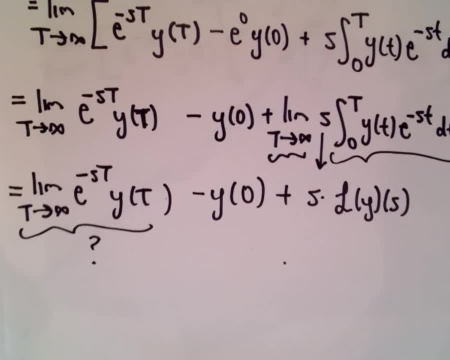 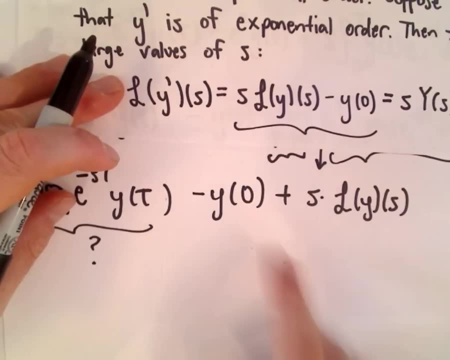 to figure out what happens to this term, and if we can show that this term goes to 0, we'll have prove in what we want. we'll have S times the Laplace transform, minus this initial condition. so our goal now is to use to show that. 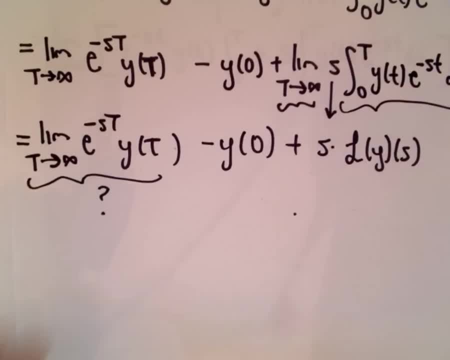 this term goes to 0. all right, well, let's see. I think we're going to have a little bit more time to think about what happens to this. we're getting getting pretty close here. what we're gonna have to use at this point now is the fact that we've got a function of exponential order. okay, so. 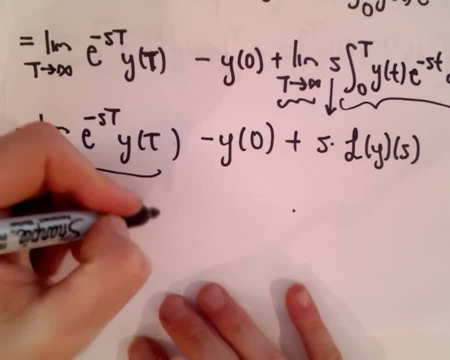 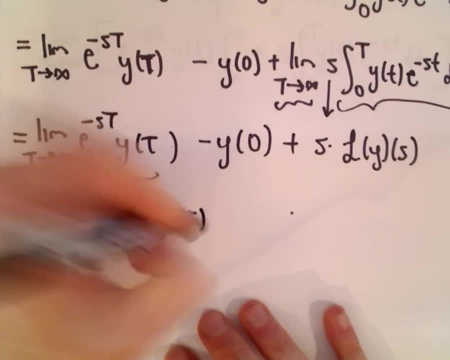 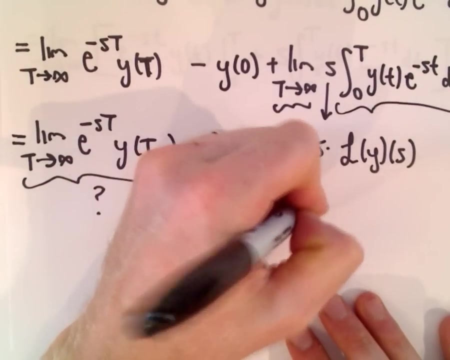 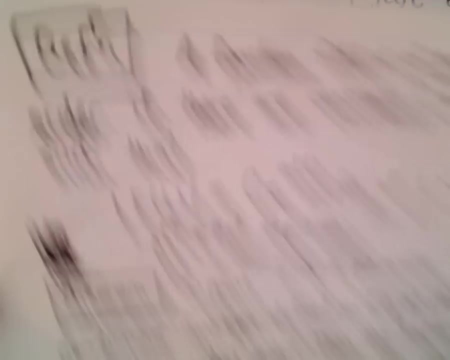 alright, so what we have here? so again, we said Y is of exponential order, so that means that Y of T, the absolute value of that, remember. that means that we can find these constants C and A, so that this happens for T greater than 0. see if I can find my exponential order definition. 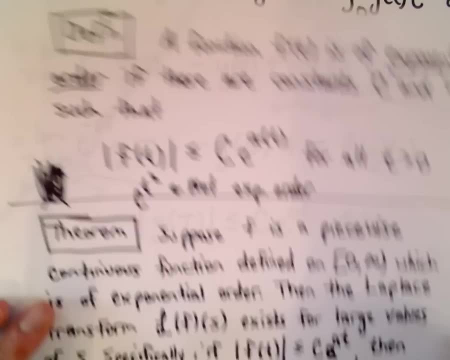 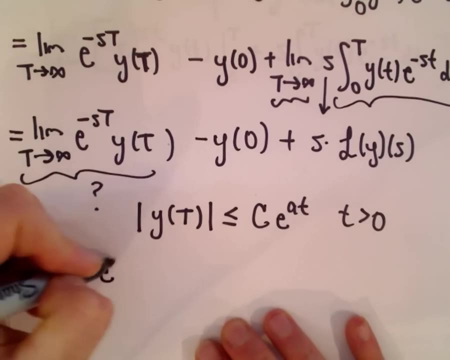 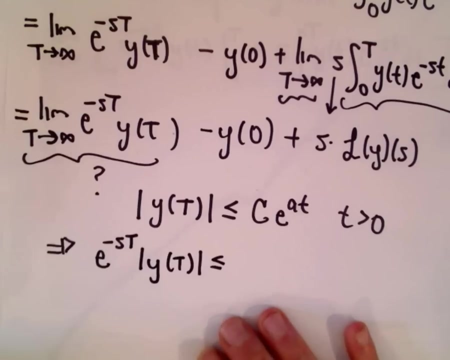 so, okay, so we're just using this property now with our function Y. okay, so that happens. well, if that happens, that means that e to the negative s T times the absolute value. okay, well, that's going to be less than or equal to e to the negative s T whoops, capital T. 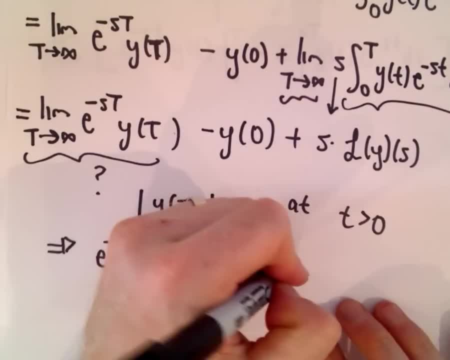 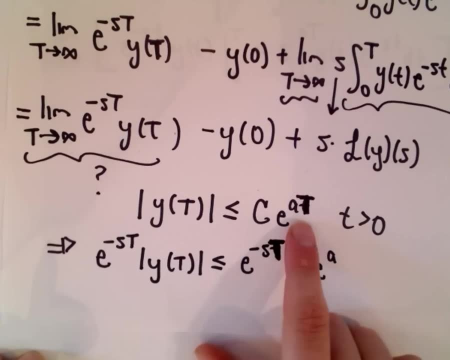 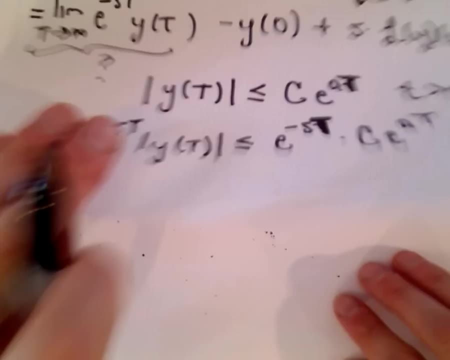 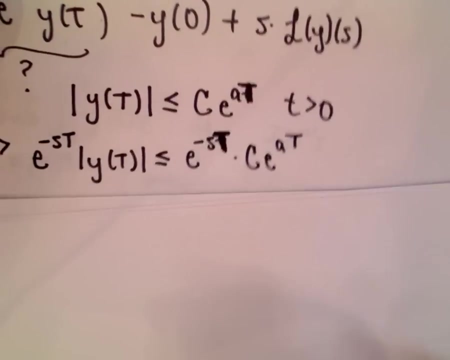 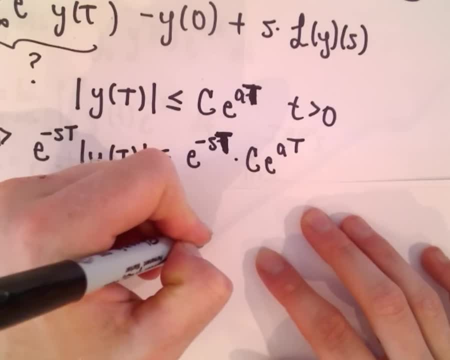 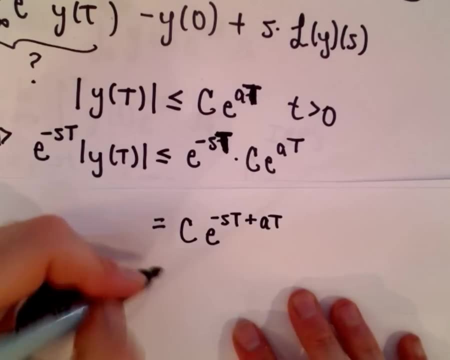 now the right side. we can simply write this: the C comes out front, we would have e, we've got like basis. so we have negative s, T plus 80 with like basis. we just add the exponents, and well, what we can do here is we can factor the. 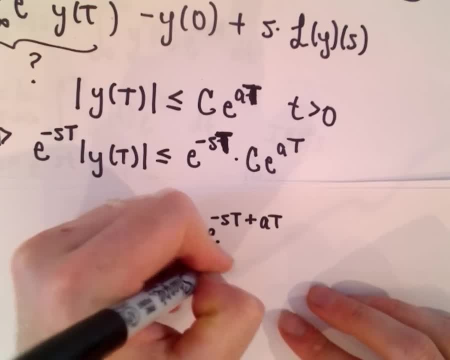 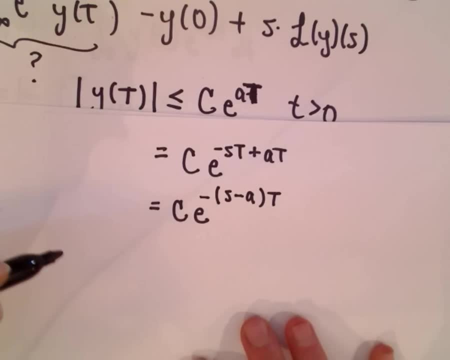 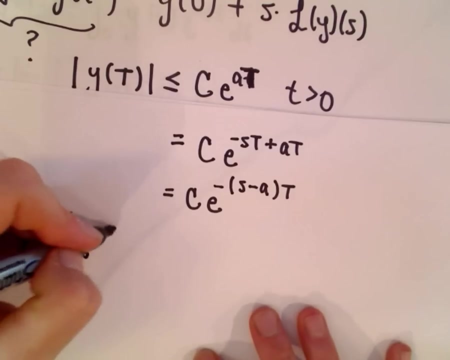 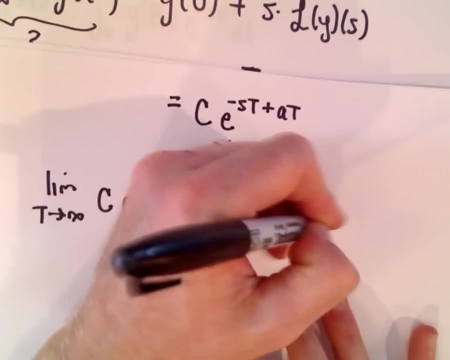 T out and we can even factor the negative out, so we would have negative s minus a times capital T. but notice, kind of the, the key thing here is okay. so if we look at the limit, as capital T goes to infinity of this term, if s is greater than a, and that was one of our, you know, one of our- results here. 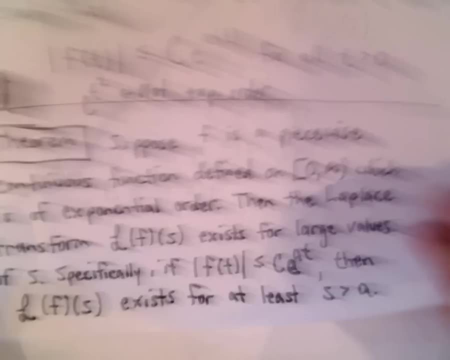 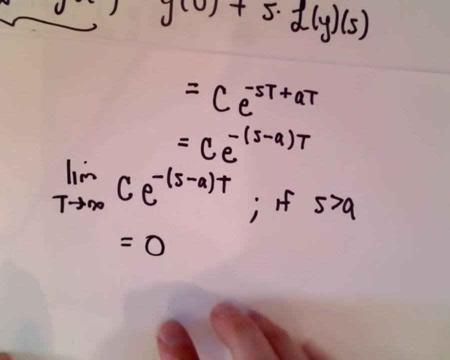 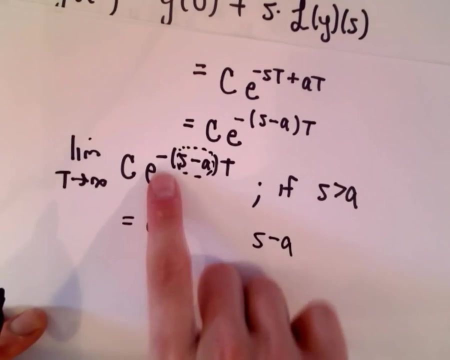 that says that's when the Laplace transform exists. okay, notice, if s is greater than a, this limit is actually going to go to well, zero. okay, you know, if s is greater than a, this is going to be some positive number, but then you have some negative. 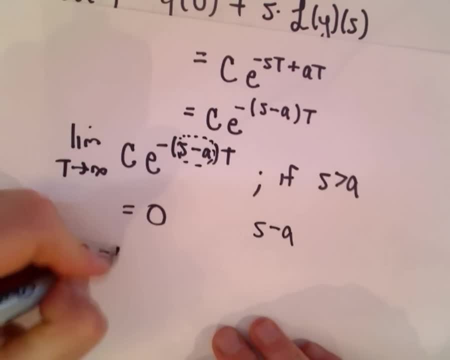 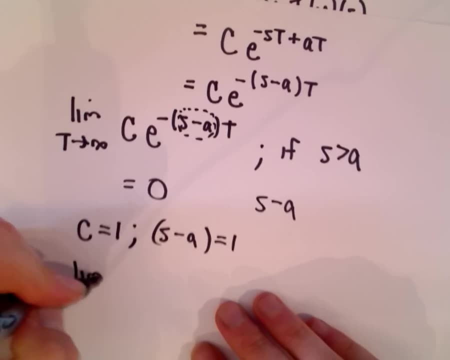 exponent attached to it. so you know, pretend, for example, that C is 1. you know, s minus a, since s is bigger than a, that's some positive number 1. well then you've got something like the limit as T goes to infinity, of e to the negative T.